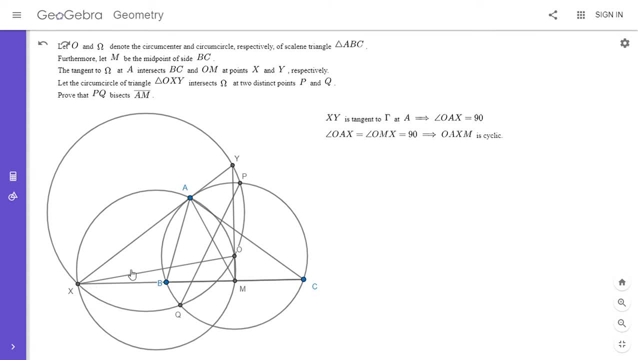 OAXM has to be a cyclic quadrilateral, Since the opposite angle is out up to 180.. All right, And now that we have three circles, I'm going to use the radical axis theorem. So it's not clear exactly yet why this would be useful. 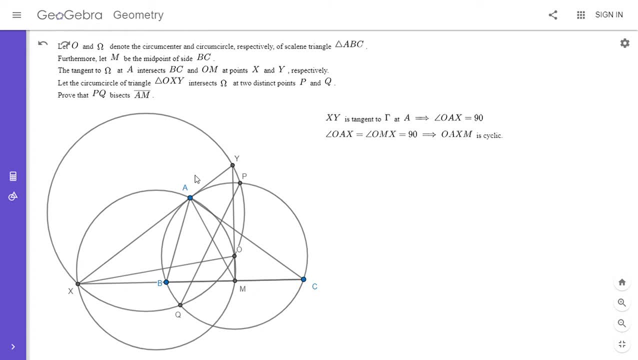 But when I was solving the problem I kind of just tried it out and it ended up helping in the end. Okay, so the three pairwise radical axes of these three circles, it's PQ, XO and the line connecting A to this other point here. 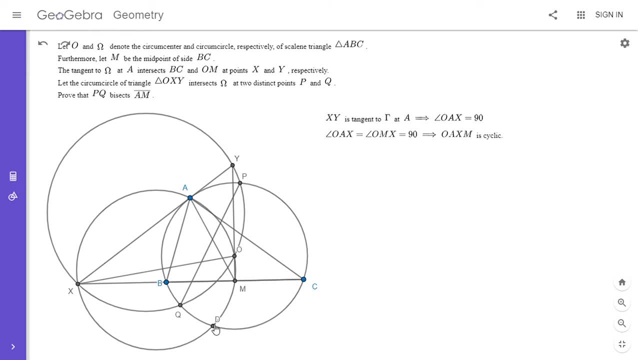 So I'm going to label this point. D is the intersection of these two circles, And so ADXO and PQ have to be concurrent by the radical axis theorem. All right, So I'm going to label that intersection point as E, All right. 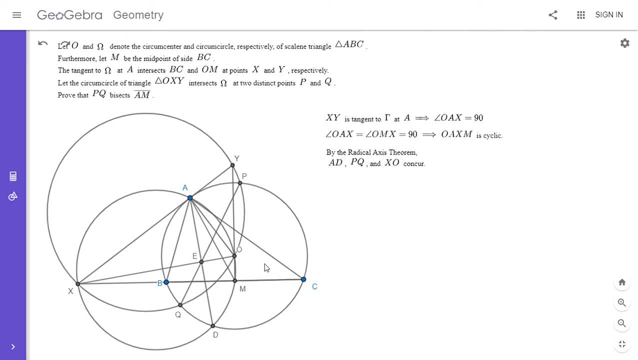 And I just drew an AO just for the heck of it. All right, All right. So what can we conclude now? So one thing I noticed is that, since AO is equal to OD, because they're both radii of the circle omega, 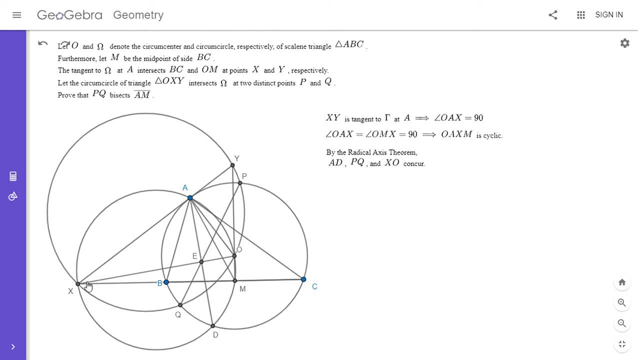 there's a symmetry about this figure, Because XO has to be a diameter of the quadrilateral AX, All right, So this circle has to have XO as a diameter, since angle OAX is 90 degrees. So I'm going to write this out. 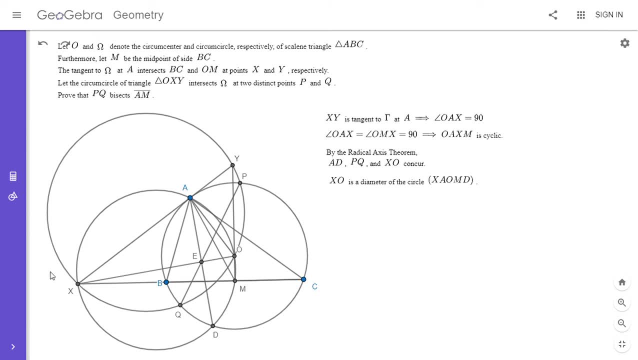 So XO is a diameter of the circle XAOMD And for those of you that don't know, when I use this notation with the brackets, it's the circle through these five points. Okay, And so if XO is a diameter and AO is equal to OD, 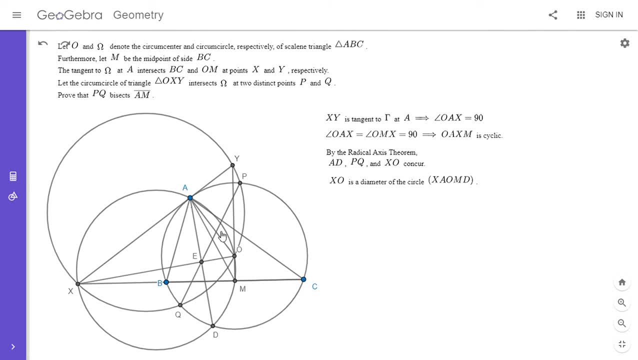 because they're both radii of gamma. then, by symmetry, D has to be the reflection of A over XO. That's fairly easy to see, Okay, So since AO is equal to OD and XO is a diameter, we have to have that D is a reflection of A over XO. 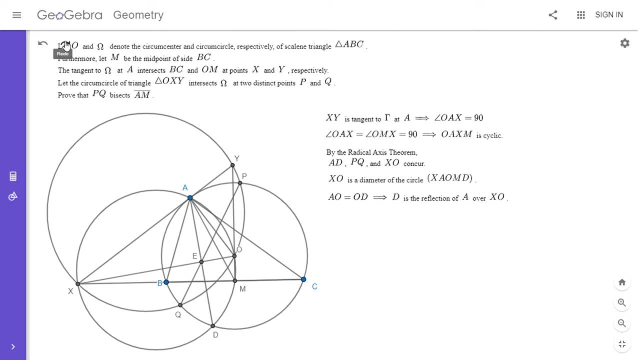 All right. So how does that help us? So here's kind of my idea And here's what I'm going to try to do to solve the problem. So if we know that D is the reflection of A over XO, then that means that AE is equal to ED. 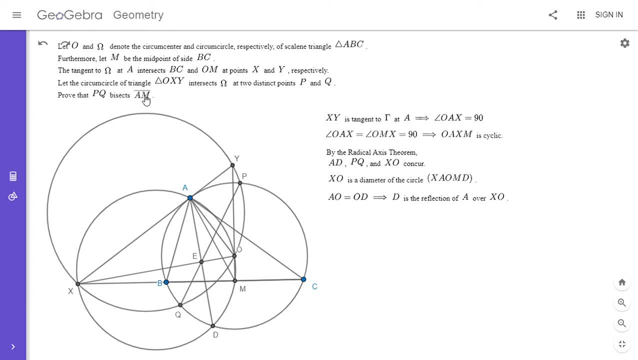 But we want to show that PQ bisects AM in the problem. So that would mean, whatever this intersection point is, let's say we called it F, we want to show that AF is equal to FM. So basically we want to show that EF is a mid-segment. 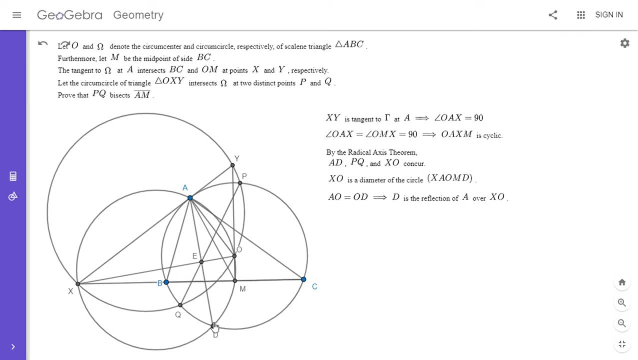 in the triangle, DAM. So what I'm actually going to do is something not that exactly, but I'm going to extend DM to meet the circle at another point. I'm going to call it F And basically, if we want to show that PQ bisects AM. 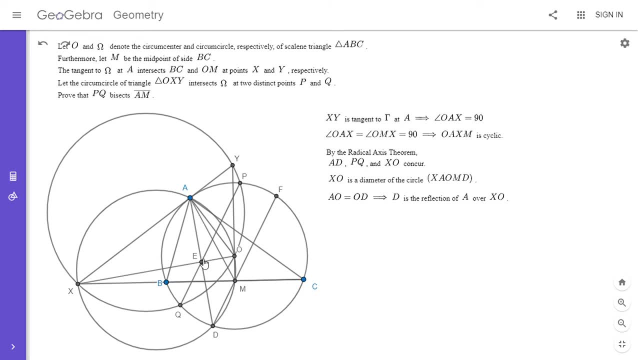 another way. so we have AE is equal to ED, As I just mentioned. But if we can show that AF and this intersection point are collinear and that this intersection point is the midpoint of AF, that would also solve the problem. So that's my strategy. 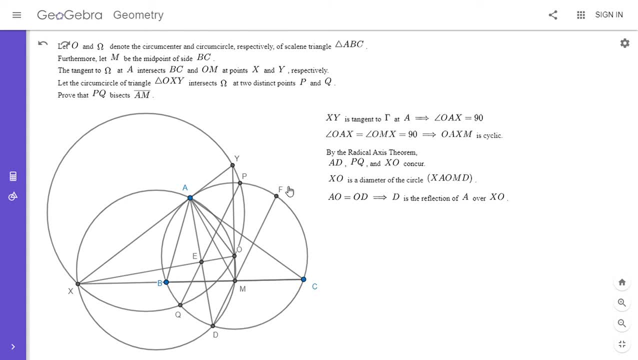 And this idea. it might seem kind of unmotivated, but I'll show you right now kind of what my motivation for this idea was. Okay, So, like I said, D is the reflection of A over XO, And so that means angle AOX is equal to angle DOX. 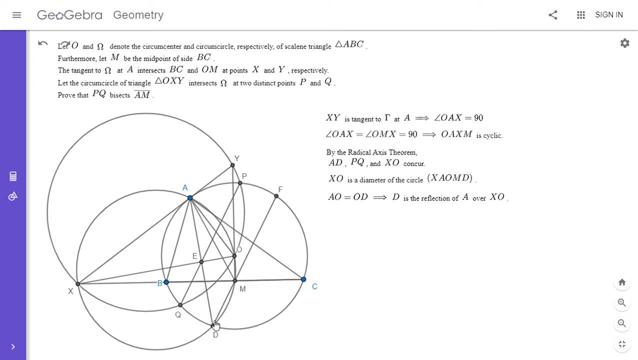 But that means it's by inscribed angles that angle AMX also has equal angle DMX because they intercept the same arcs. So I'm going to write this out here For now. I'm letting H denote this intersection point. So we have: angle AMX is equal to angle AOX. 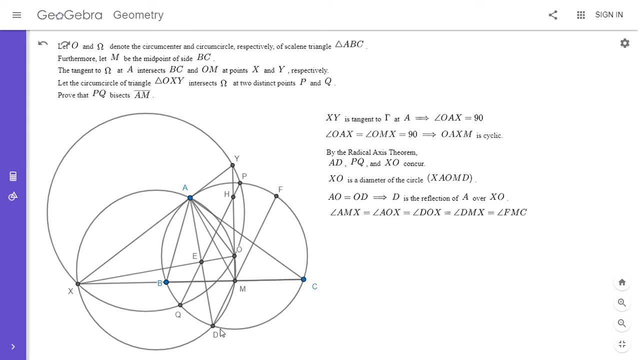 is equal to angle DOX using this reflection And angle DOX is equal to angle DMX. So angle AMX is equal to angle DMX And angle DMX is equal to angle FMC. All right, So we have, if angle AMX is equal to angle FMC. 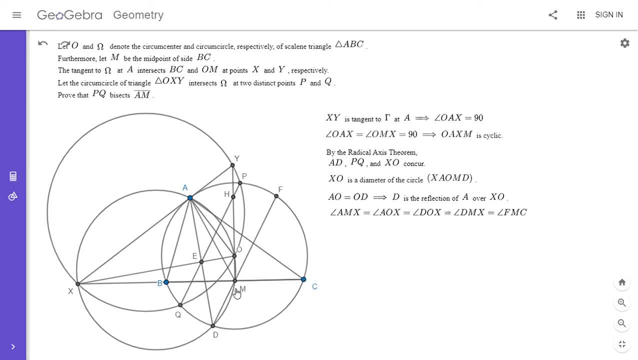 there's a certain symmetry in the figure here, because M is the midpoint of BC and OM is clearly perpendicular to BC. So if we have angle AMB, because AMX is the same as AMB, if angle AMB is equal to angle FMC. 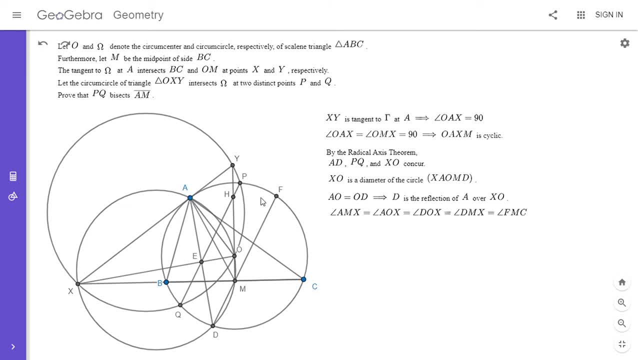 by symmetry, F has to be the reflection of A, And if angle AMX is equal to angle DMX, it's the reflection of A. So my motivation for extending DM to meet the circle of point F was that I realized that angle AMX 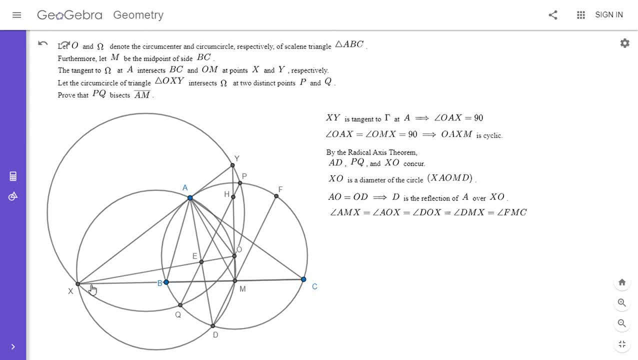 is equal to angle DMX. So that was my motivation for it. If you're curious, but we know that F is the reflection of A over MY, then because angle AMX is equal to angle FMC, So it's easy enough. C, So it's easy to see that by symmetry, Alright, And, like I mentioned, if we can show that, 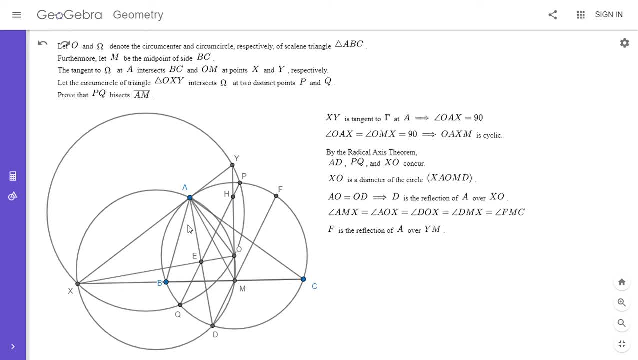 H is the midpoint of AF and E is the midpoint of AD, then by symmetry, that would mean that HE would have to be a midsegment in the triangle ADF, And so that would mean that HE would bisect AM, which would solve the problem. So that's our goal. We want to show that H. 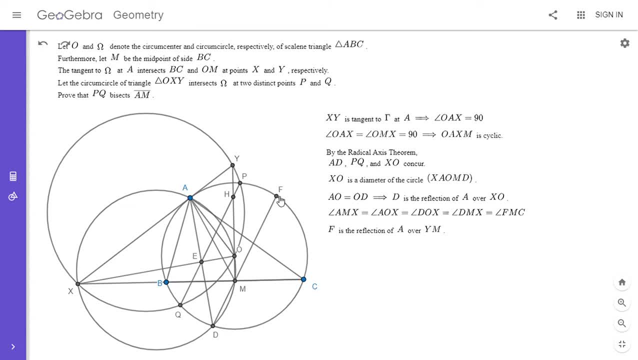 is the midpoint of AF. So how do we do that? And this is a little clever, but I'm actually going to use the Radical Axis Theorem again. Ok, so f is the reflection of A over yM. so how do we use that fact? Well, we know that angle is 90 degrees, And so therefore, 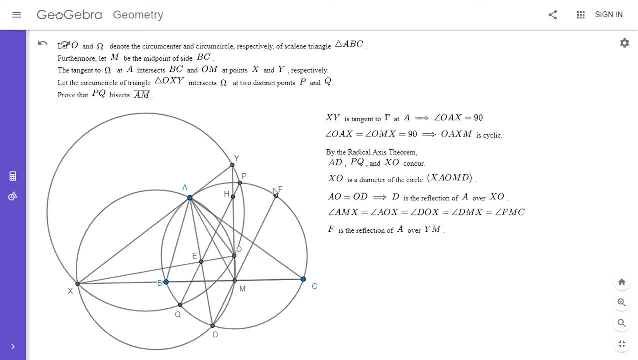 angle • vimos. Итак h-o по У-a我們的 ис predicted could be z ​​prime probing x س�� ". FO also has to be 90 degrees, and so YAOF has to be cyclic. All right, so I'm going to write that. 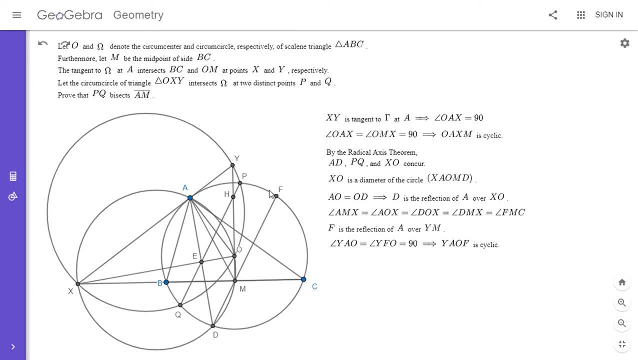 out. So angle YAO is equal to angle YFO and they're both 90 degrees. So since the opposite angles add up to 180, YAOF has to be a cyclic quadrilateral. so we can draw the circle through those four points. And now we can apply the radical axis theorem again, and it gets us. 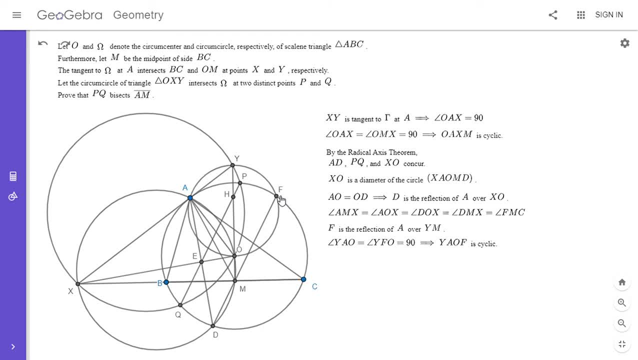 exactly what we want- that A, H and F are collinear. So I'm going to show you how I do that right here. So we have the three circles: YAOF, so this is the bracket notation, so the circle through YAO and F. Then we have another circle here through a lot of different points. 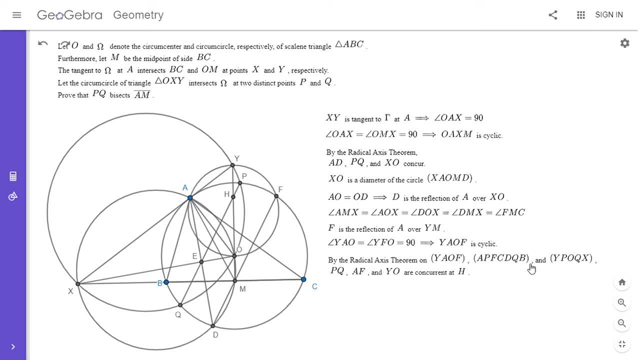 the circle through APF, C, D, Q and B, And then we also have this biggest circle, YPOQX. Okay, and if we use the radical axis theorem on those three circles? so I kind of got a little. 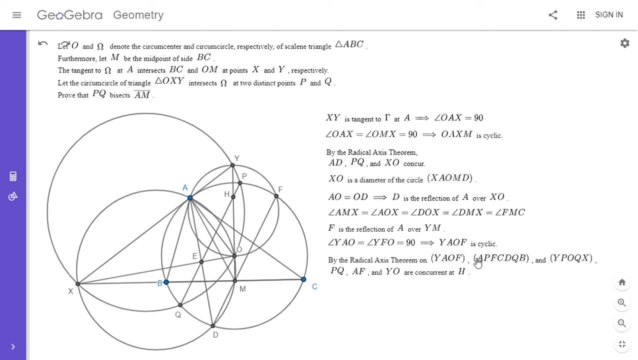 lucky here, but it gives us exactly what we want. So it's pretty convenient when we have all the letters written out like this, because it's easy to see what the radical axes are. So if you look at this circle and this circle, what two letters do they share in common? They both have an A. 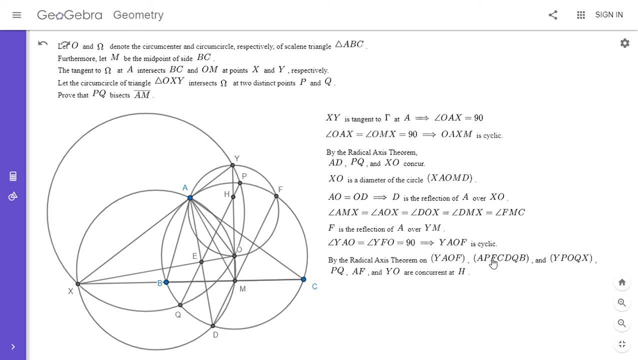 and they both have an F. So AF is one of the radical axes. and if we look at this and this, so these last two circles, they both share P and Q, so PQ is another radical axis. And then if we take the first and last circle, so we have YAOF and YPOQX and we 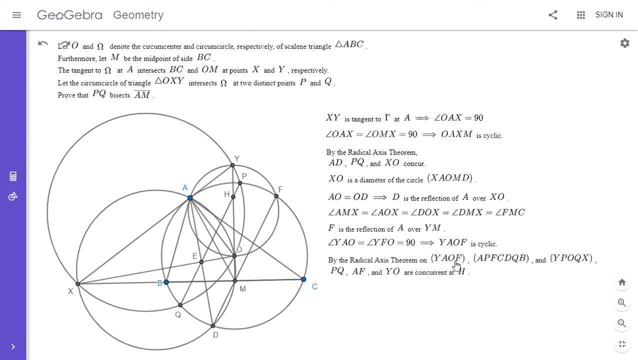 look at the two letters that those have in common: it's Y and O, So YO is the third radical axis, and so devices O and O have to be concurrent, but P, Q and YO meet a point H, So that's the. 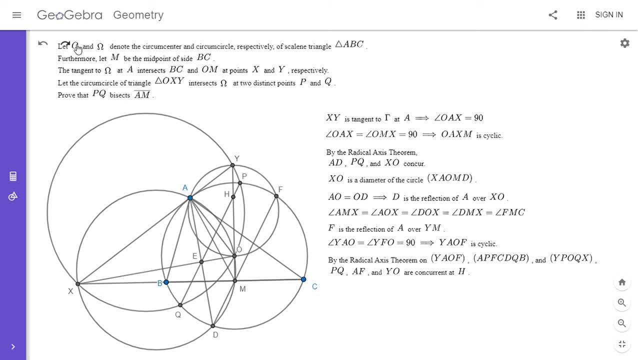 thing that AF has to pass through H, So we can draw that segment. All right, and now we're essentially there, because we said that F is the reflection of A over YM. So that means that AH has to equal HF. okay, Because that's the only way that F could reflect H. Okay so,